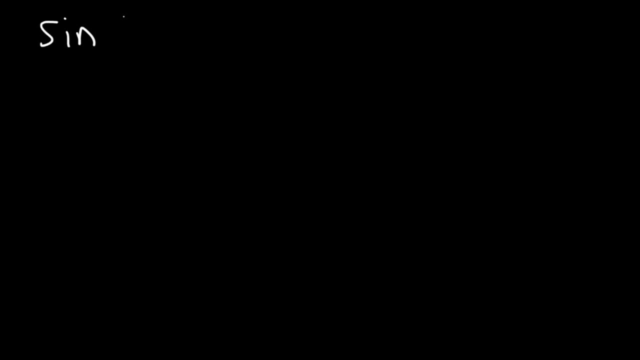 So if you saw a terrible looking expression like this, what would you do? So what is sine of 2 arc cosine 4 over 5?? So notice that we need to use the double angle formula. By the way, just to review something: sine of an angle is equal to a value. 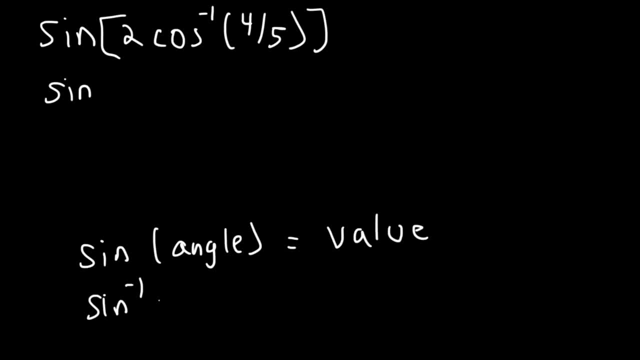 So arc sine or arc cosine of a value is equal to an angle. Make sure you understand this. So when you see arc cosine of something that's equal to an angle, So what we really have is sine 2 theta, where theta is actually arc cosine 4 over 5.. 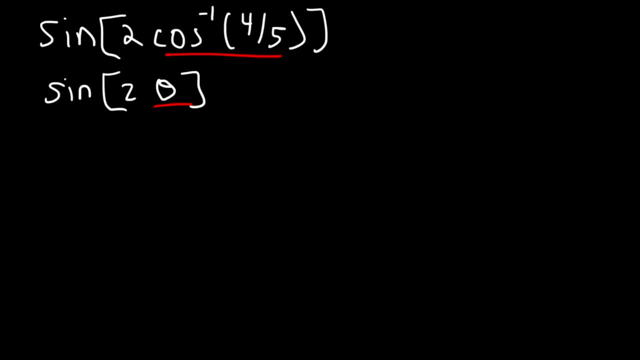 So the arc of any type of trig function is always equal to an angle, which you can call theta, alpha or beta. So in this example theta is arc cosine 4 over 5.. So that means that cosine theta is 4 over 5.. 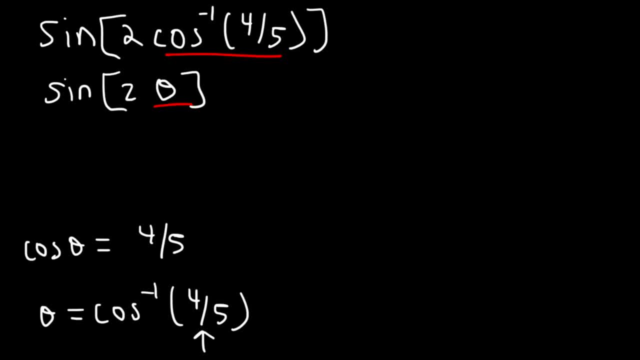 Arc cosine is positive in quadrant 1.. It's negative in quadrant 2.. And arc cosine does not exist in quadrants 3 and 4.. So therefore we have a right triangle in quadrant 1.. Cosine is adjacent divided by hypotenuse. 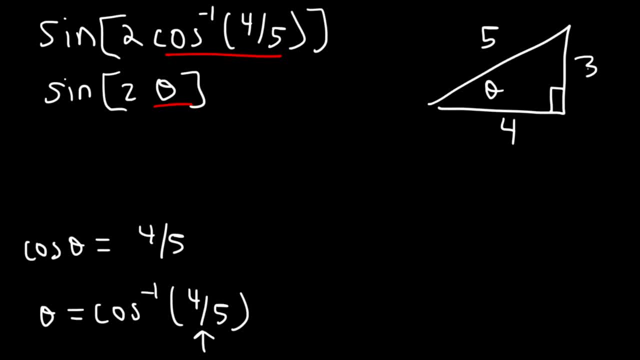 So the missing side is 3.. This is the 3,, 4, 5 right triangle. So now we can find the value of sine theta. Sine theta is opposite over hypotenuse, So it's 3 over 5.. 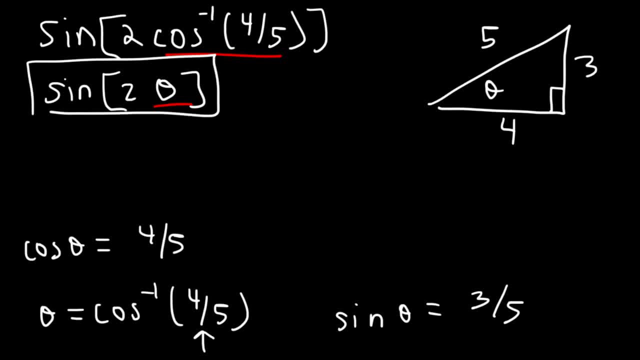 So now we can evaluate sine 2 theta Using the double angle formula, which is 2 sine theta, cosine theta. So we said that sine theta is 3 divided by hypotenuse And cosine theta is 4 over 5.. 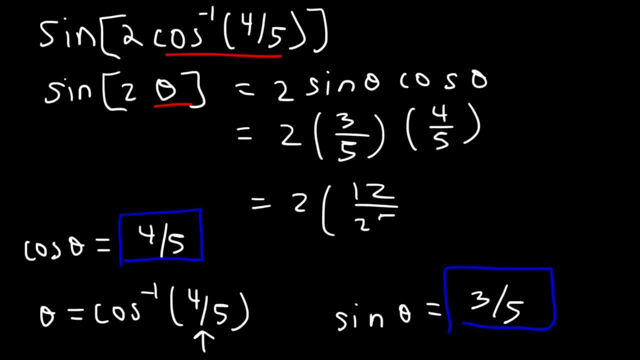 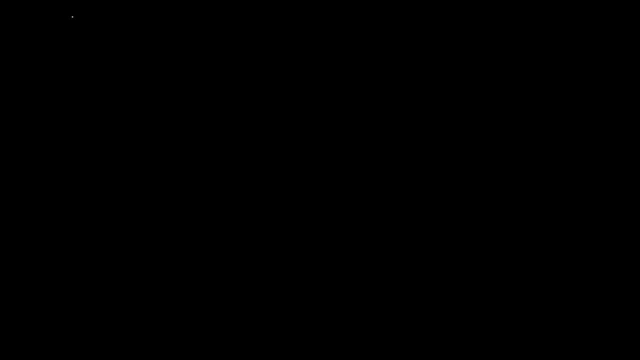 3 times 4 is 12.. 5 times 5 is 25.. 2 times 12 is 24.. So the answer is 24 over 25.. Here's one you could try: Cosine of 2 arc tangent negative, 12 over 5.. 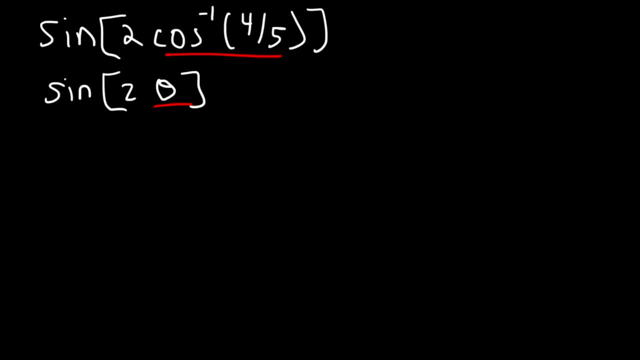 So the arc of any type of trig function is always equal to an angle, which you can call theta, alpha or beta. So in this example theta is arc cosine 4 over 5.. So that means that cosine theta is 4 over 5.. 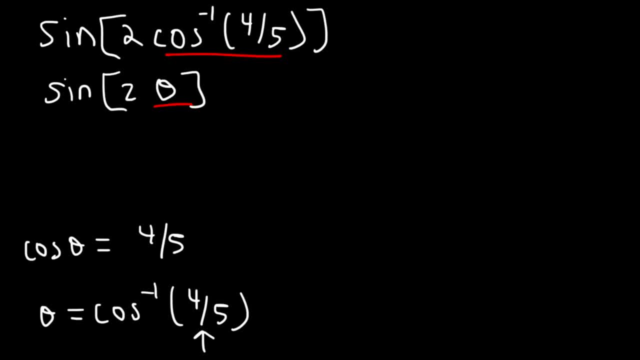 Arc cosine is positive in quadrant 1.. It's negative in quadrant 2.. And arc cosine does not exist in quadrants 3 and 4.. So therefore we have a right triangle in quadrant 1.. Cosine is adjacent divided by hypotenuse. 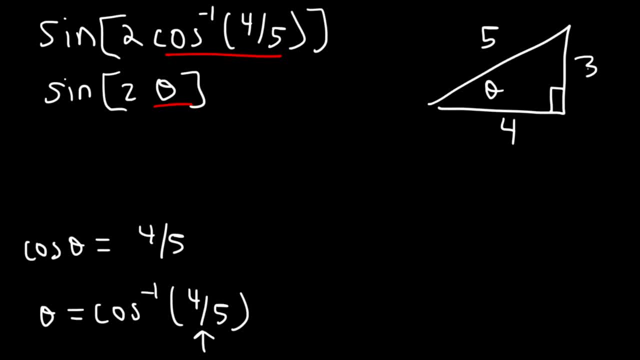 So the missing side is 3.. This is the 3,, 4, 5 right triangle. So now we can find the value of sine theta. Sine theta is opposite over hypotenuse, So it's 3 over 5.. 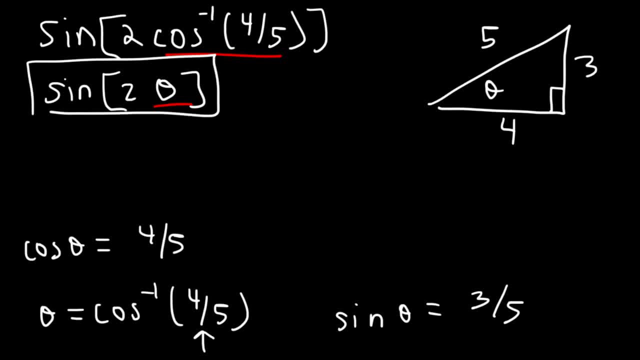 So now we can evaluate sine 2 theta Using the double angle formula, which is 2 sine theta, cosine theta. So we said that sine theta is 3 divided by hypotenuse And cosine theta is 4 over 5.. 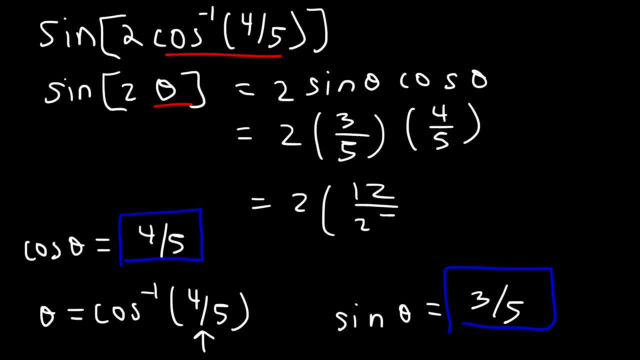 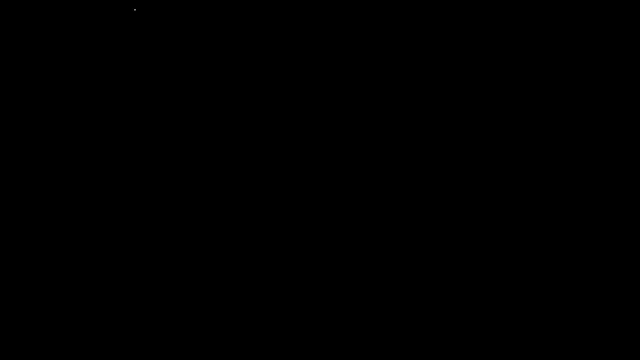 3 times 4 is 12.. 5 times 5 is 25.. 2 times 12 is 24.. So the answer is 24 over 25.. Here's one you could try: Cosine of 2 arc tangent negative, 12 over 5.. 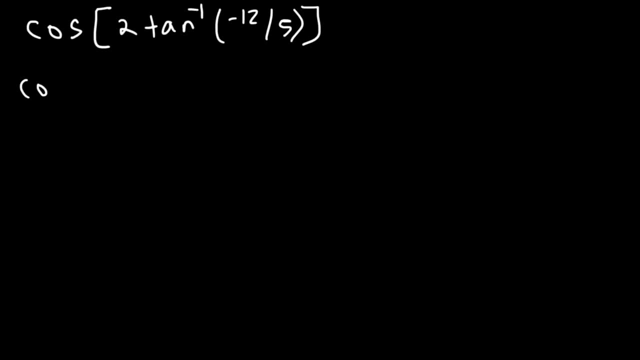 Go ahead and simplify that. So we're looking for cosine of 2 theta. So you need to realize that theta is actually arc tan of negative 12 over 5.. So if theta is equal to that expression, then we could say that tangent of theta is negative 12 over 5.. 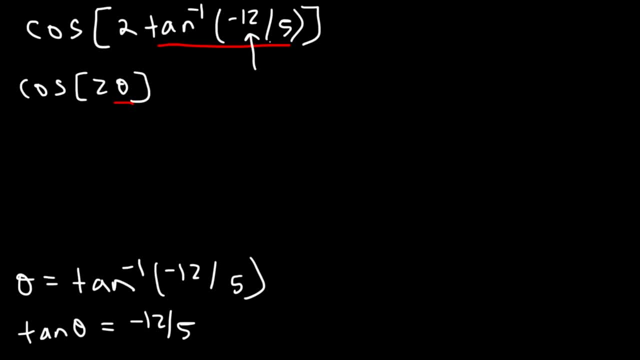 Now arc tan only exists in quadrants 1 and 4. So because we have a negative value, we need to draw the right triangle in quadrant 4.. Tangent is opposite over adjacent, So adjacent is positive 5.. 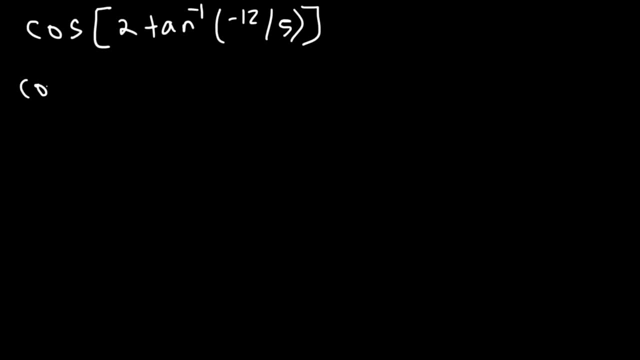 Go ahead and simplify that. So we're looking for cosine of 2 theta. So you need to realize that theta is actually arc tan of negative 12 over 5.. So if theta is equal to that expression, then we could say that tangent of theta is negative 12 over 5.. 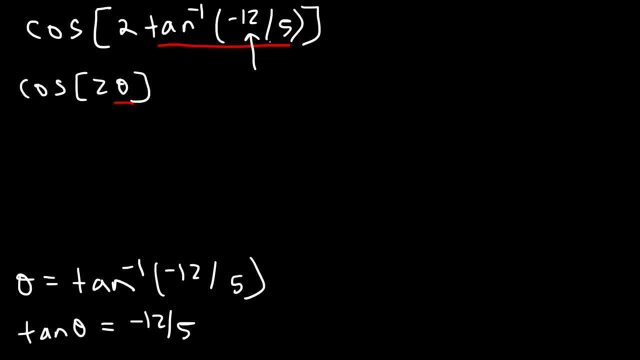 Now arc tan only exists in quadrants 1 and 4.. So because we have a negative value, we need to draw the right triangle. So we're going to draw the right triangle in quadrant 4.. Tangent is opposite over adjacent. 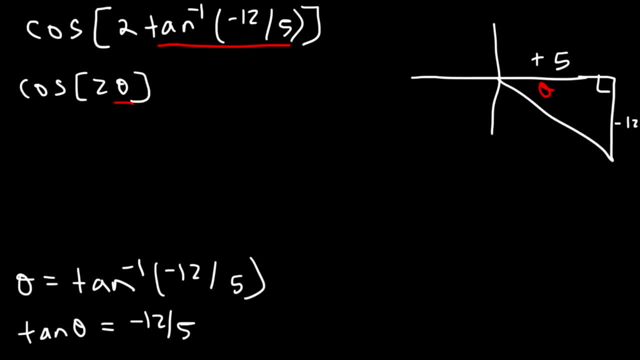 So adjacent is positive, 5. Opposite is negative, 12. X is positive in quadrant 4.. But Y is negative in quadrant 4. And what we have is the 5,, 12, 13 right triangle. So now let's find sine and cosine. 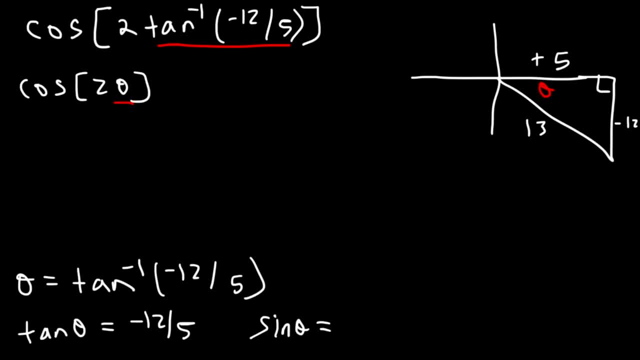 So sine theta of that triangle is equal to the opposite side divided by the hypotenuse. So that's negative 12 over 13.. Cosine theta is adjacent over hypotenuse, So cosine is 5 over 13.. 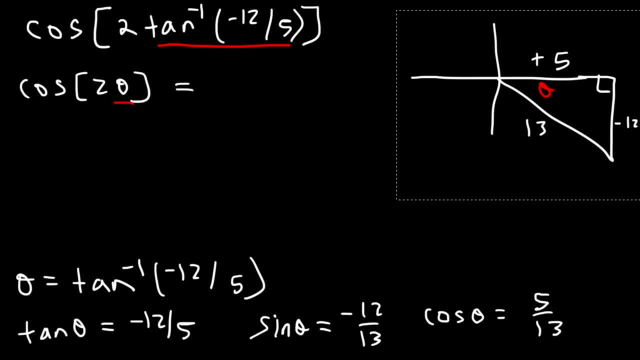 Now let's use the double angle formula for cosine 2 theta. So I'm going to use cosine squared minus sine squared. So I'm going to use cosine squared minus sine squared. So cosine, that's 5 divided by 13.. 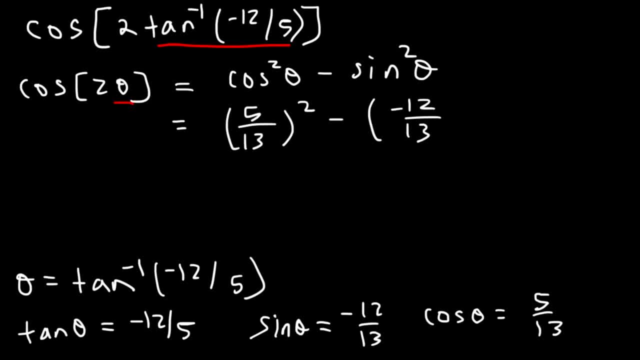 And sine is negative: 12 over 13.. 5 squared is 25.. 13 squared is 169.. Negative 12 squared is positive, 144.. But there's a negative in front And this we're going to have the same denominator. 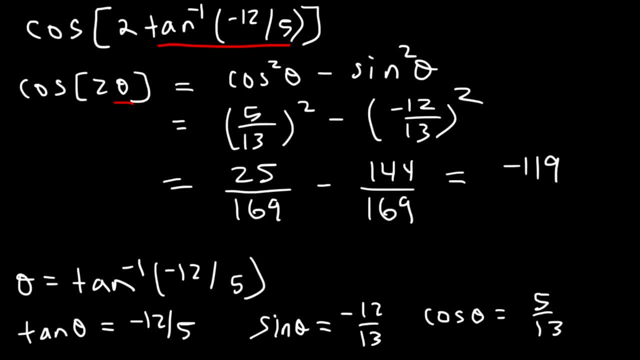 Now, 25 minus 144 is negative 119.. So therefore, this is the answer: Cosine 2, theta, which is cosine arc, I mean cosine 2, arc tangent, all of that, all of that is equal to negative 119 over 169.. 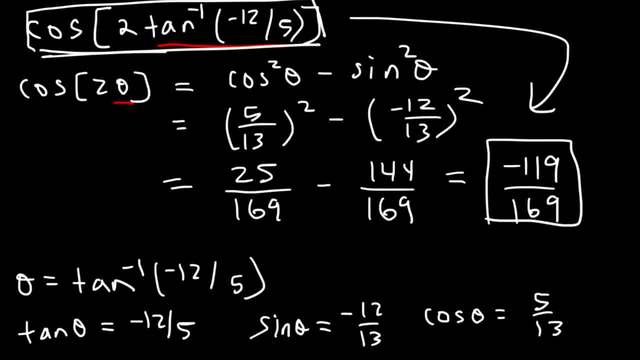 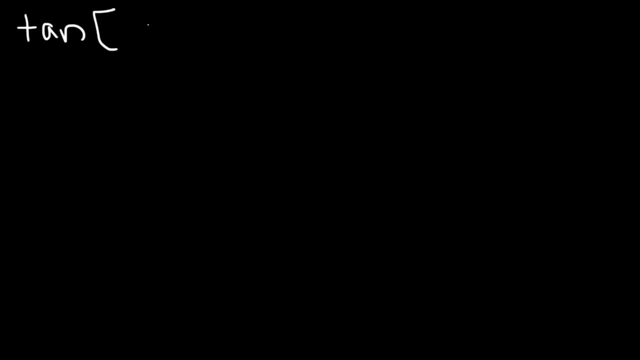 So that's the final answer. So when you see this, basically you're looking for the value of cosine 2 theta. Now let's try a problem with tangent. What is tan of 2 arc cosine negative 8 over 17?? 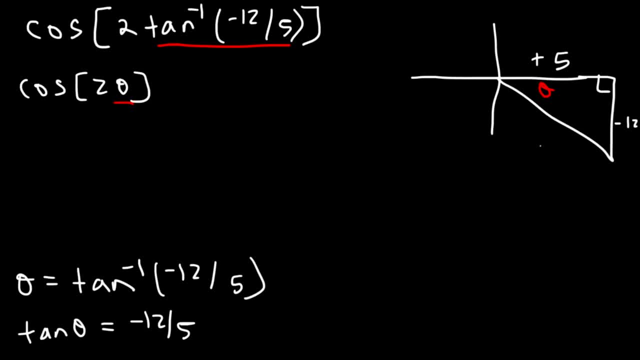 Opposite is negative 12.. X is positive in quadrant 4.. But Y is negative in quadrant 4.. And what we have is the 5,, 12,, 13 right triangle. So now let's find sine 2 theta. 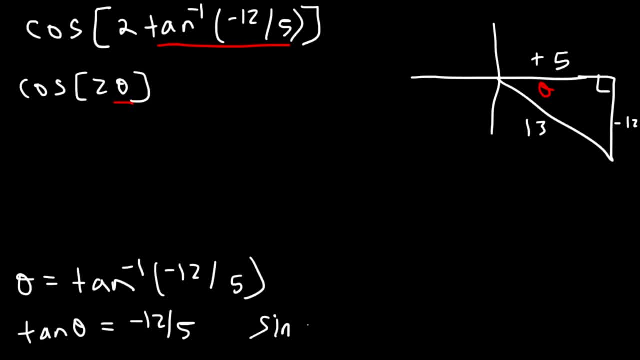 Sine and cosine. Sine theta of that triangle is equal to the opposite side divided by the hypotenuse, So that's negative 12 over 13.. Cosine theta is adjacent over hypotenuse, So cosine is 5 over 13.. 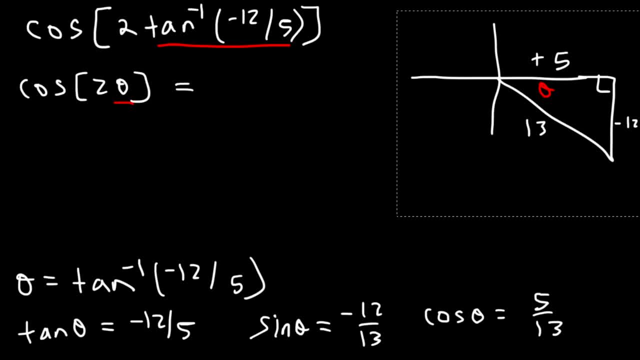 Now let's use the double angle formula for cosine 2 theta. So I'm going to use cosine squared minus sine. So cosine, that's 5 divided by 13. And sine is negative: 12 over 13.. 5 squared is 25.. 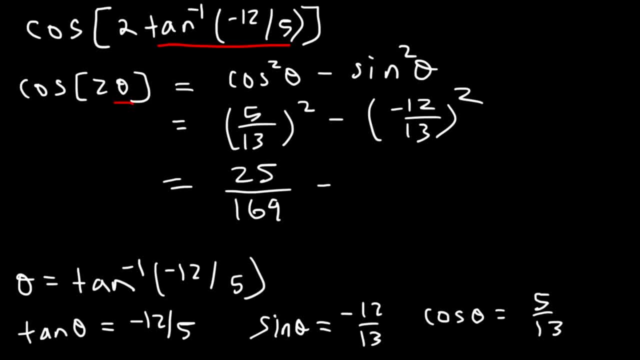 13 squared is 169.. Negative 12 squared is positive 144.. But there's a negative in front And this we're going to have the same denominator Now: 25 minus 144 is negative 119.. So therefore, this is negative: 12 over 13.. 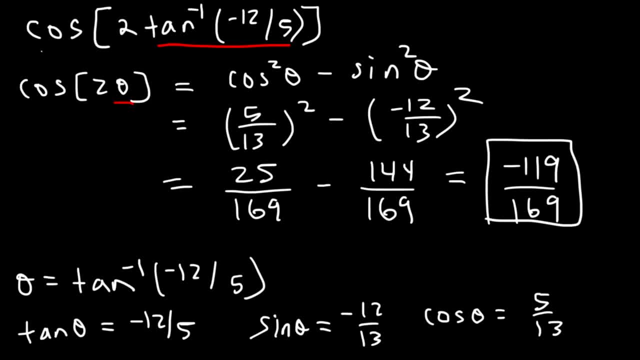 So therefore, this is the answer: Cosine 2 theta, which is cosine 2 arc tangent, all of that, All of that is equal to negative 119 over 169.. So that's the final answer. So when you see this, basically you're looking for the value of cosine 2 theta. 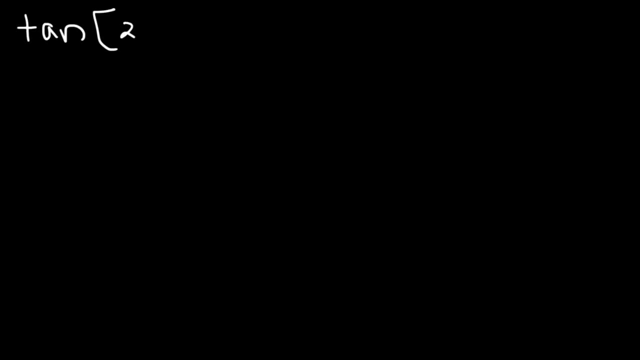 Now let's try a problem with tangent. What is tan of 2 arc cosine negative 8 over 17?? So take a minute and try this problem. So once again we're looking for tangent of 2 theta. So theta in this problem is arc cosine negative 8 over 17.. 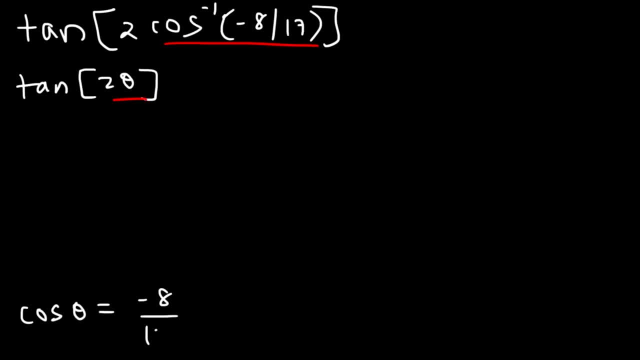 Which means that cosine theta is negative, 8 over 17.. Arc cosine is negative in quadrant 2.. So that's where we're going to draw the triangle. Cosine is adjacent divided by hypotenuse. So this is the 8,, 15, 17 triangle. 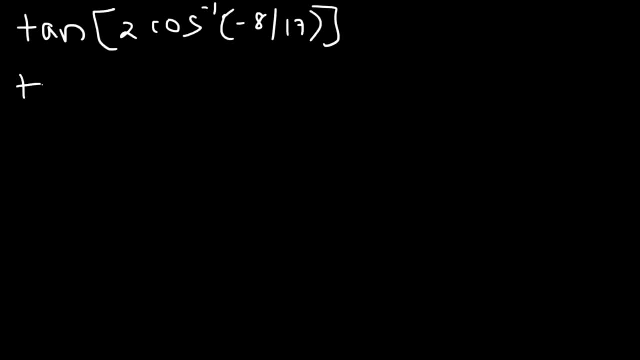 So take a minute and try this problem. So once again we're looking for tangent of 2 theta. So theta in this problem is arc cosine negative 8 over 17.. Which means that cosine theta is negative 8 over 17.. 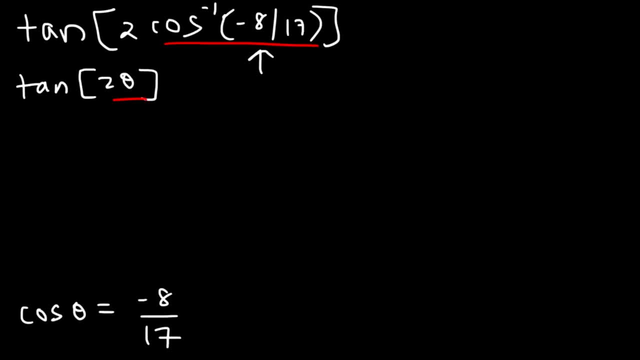 Arc cosine is negative in quadrant 2.. So that's where we're going to draw. the triangle Cosine is adjacent divided by hypotenuse. So this is the 8,, 15,, 17 triangle. X is negative in quadrant 2.. 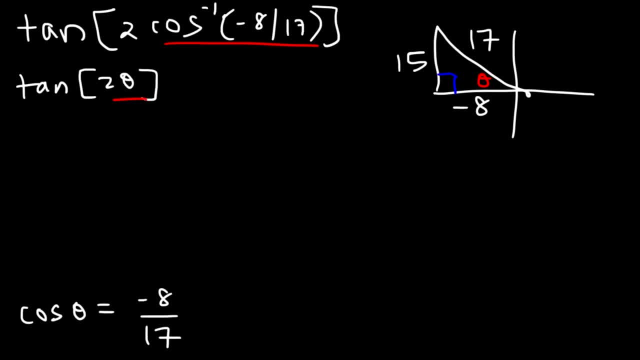 Y is positive. Now we don't need to find sine theta. All we need to find in this triangle is tangent 1 theta. So tan theta is opposite over hypotenuse. I mean, excuse me, So it's opposite over adjacent. 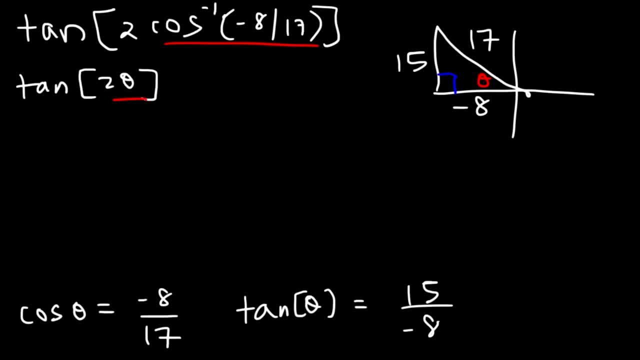 So it's 15 divided by negative 8.. Now let's use the formula for tan 2 theta. Tan 2 theta is 2 tangent theta divided by 1 minus tan squared. So now let's replace tangent with 15 over negative 8.. 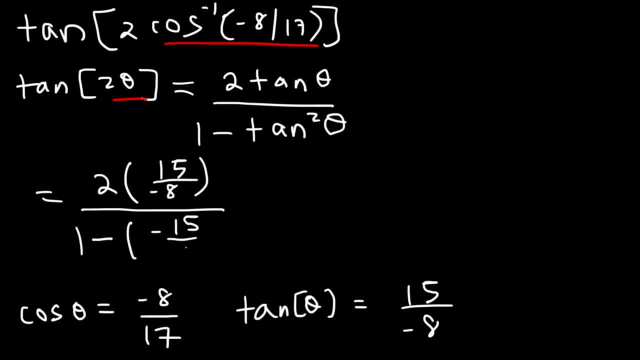 So we have 1 minus negative 15 over 8. squared Now 2 times 15 is 30. So we have negative 30 over 8 on top. On the bottom, negative 15 squared is positive 225.. 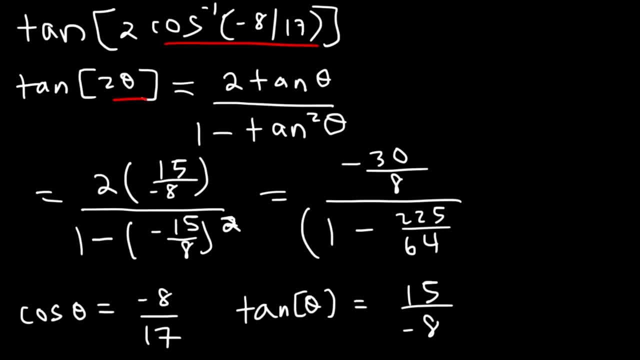 And 8 squared is 64. So let's multiply the top and bottom by 64.. On top, I'm going to write it as 8 times 8, which is equivalent to 64. So I can cancel one of the 8's. 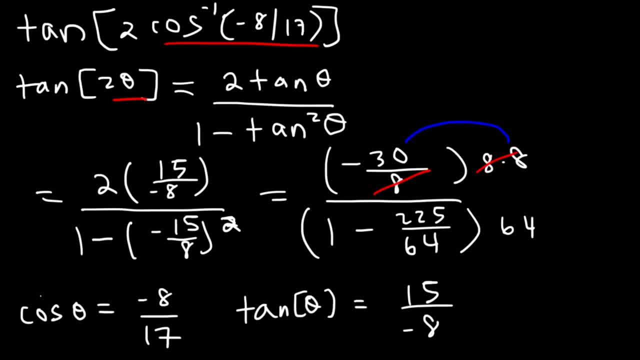 So what I have left over is 8 times negative 30,, which is negative 240.. On the bottom I have 64 times 1, and then 225 over 64. These cancel. I'm just going to have 225.. 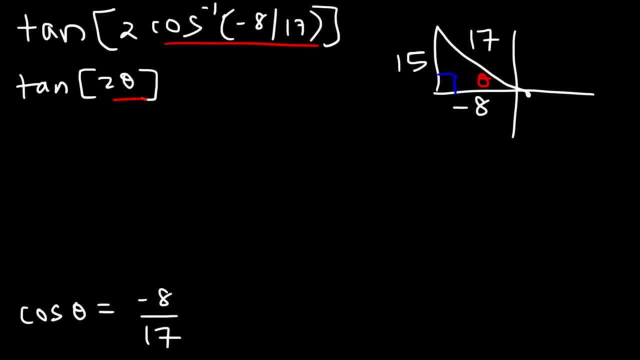 X is negative in quadrant 2.. Y is positive. Now we don't need to find sine theta. All we need to find in this triangle is tangent 1 theta. So tan theta is opposite. over hypotenuse. I mean, excuse me, 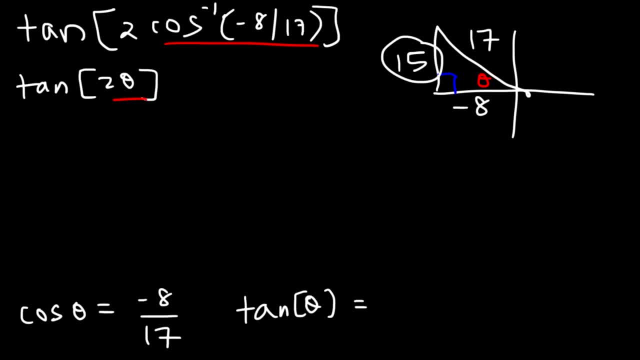 So it's opposite over adjacent. So it's 15 divided by negative 8.. Now let's use the formula for tan 2 theta. Tan 2 theta is 2 tangent theta divided by 1 minus tan squared. So now let's replace tangent with 15 over negative 8.. 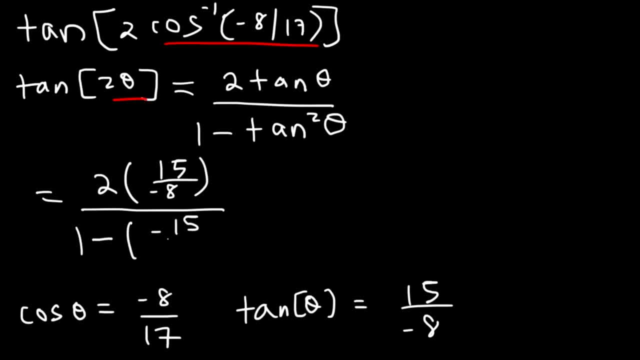 So we have 1 minus negative 15 over 8. squared Now 2 times 15 is 30. So we have negative 30 over 8 on top. On the bottom, negative 15 squared is positive 225.. 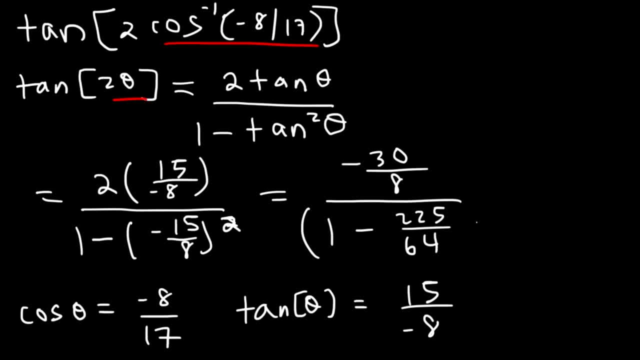 And 8 squared is 64. So let's multiply the top and bottom by 64.. On top, I'm going to write it as 8 times 8, which is equivalent to 64.. So I can cancel one of the 8s. 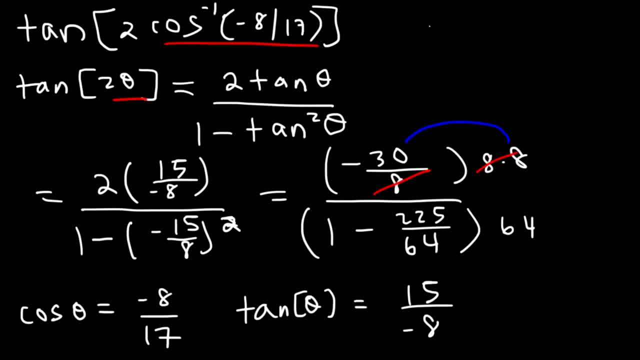 So what I have left over is 8 times negative 30,, which is negative 240.. On the bottom I have 64 times 1. And then 225 over 64.. These cancel And I'm just going to have 225.. 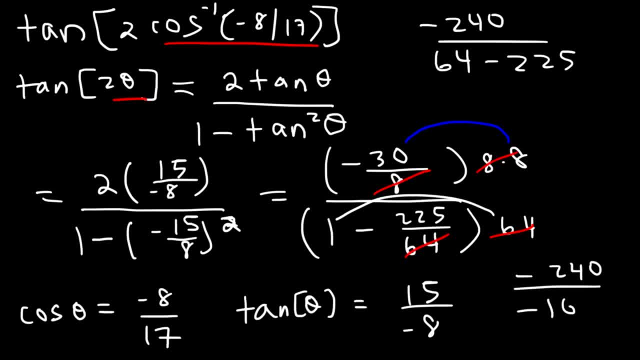 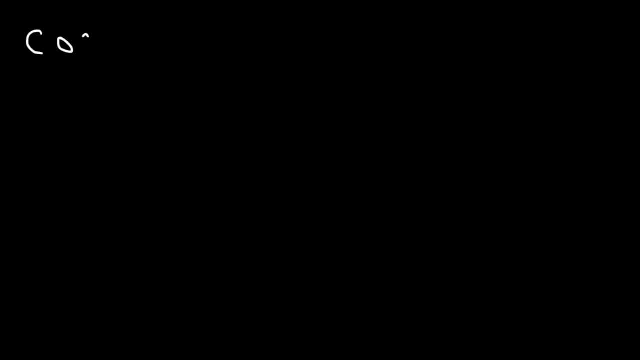 64 minus 225 is negative 161.. So the final answer is positive 240 over positive 161.. So that's equal to this entire thing. Let's try a different problem: Cosine squared of 1, half arc sine 4 over 5.. 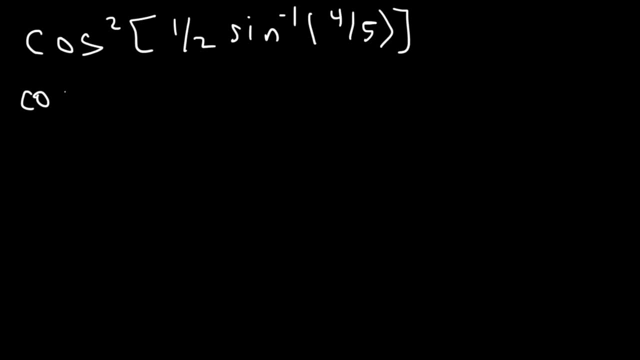 Go ahead and simplify this expression. So this is cosine squared of 1 half times theta. So an arc trig value is always equal to an angle. So arc sine 4 over 5.. Is theta? So if theta is arc sine 4 over 5, then that means that sine theta is 4 over 5.. 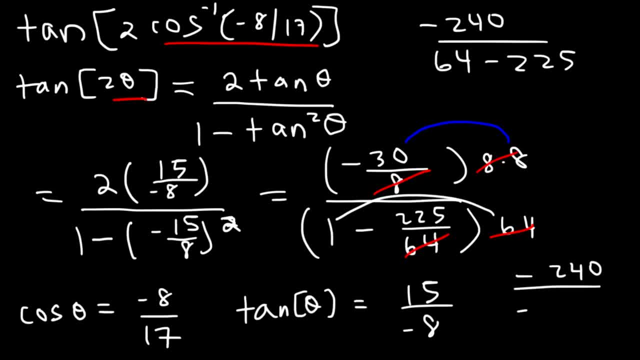 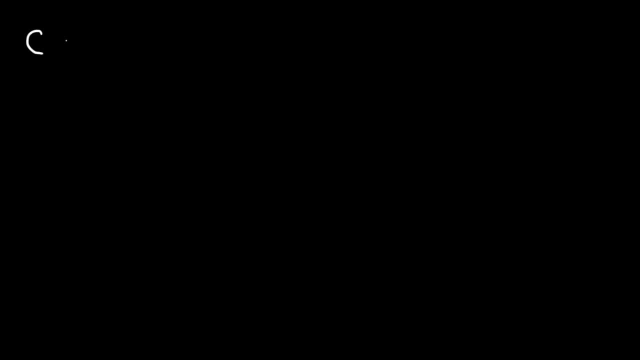 64 minus 225 is negative 161.. So the final answer is positive 240 over positive 161.. So that's equal to this entire thing. Let's try a different problem: Cosine squared of 1 half arcsine 4 over 5.. 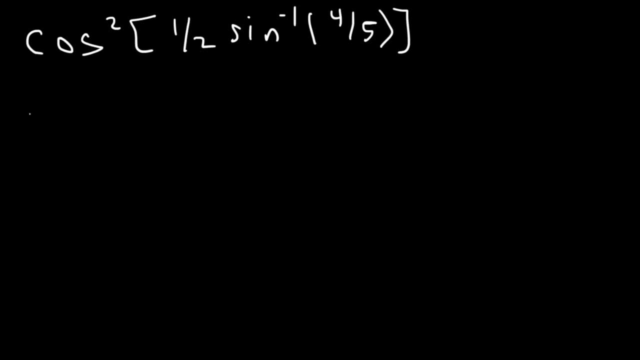 Go ahead and simplify this expression. So this is cosine squared of 1 half times theta. So an arc trig value is always equal to an angle, So arcsine 4 over 5.. is theta? So if theta is arcsine 4 over 5, then that means that sine theta is 4 over 5.. 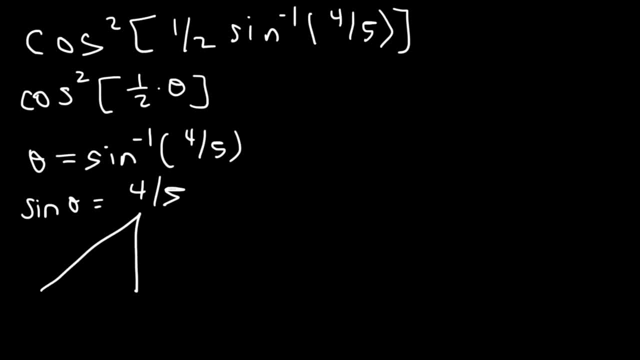 And arcsine is positive in quadrant 1.. So we have a right triangle in quadrant 1, and sine is opposite over hypotenuse. The missing side is 3.. Now we need the value of cosine theta. Okay, cosine is adjacent over hypotenuse, So cosine theta is 3 over 5, and we'll use this soon. 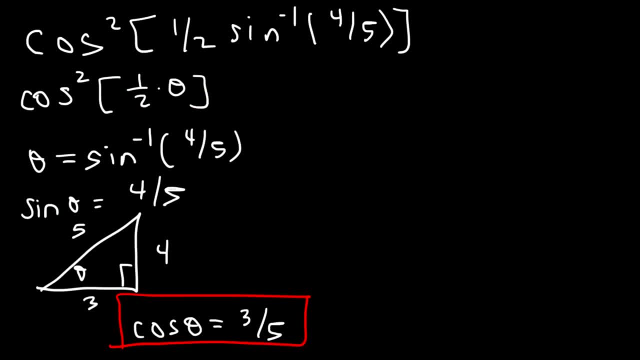 So right now we need to use the half angle formula or we can use the power reducing formula. Now we know that cosine squared theta is 1 plus cosine 2 theta divided by 2.. So if we divide this angle by half and get cosine squared, 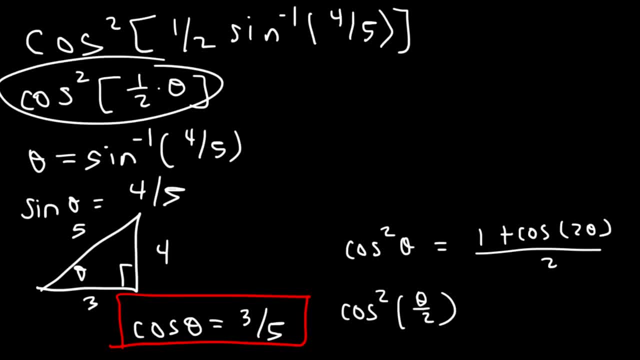 theta over 2, which is what we have here- then all we're going to do is divide this angle by half. I mean not by half, but by 2.. So that will be 1 plus cosine theta over 2.. And this is the equation that we need to use. So 1 plus cosine theta divided by 2,. 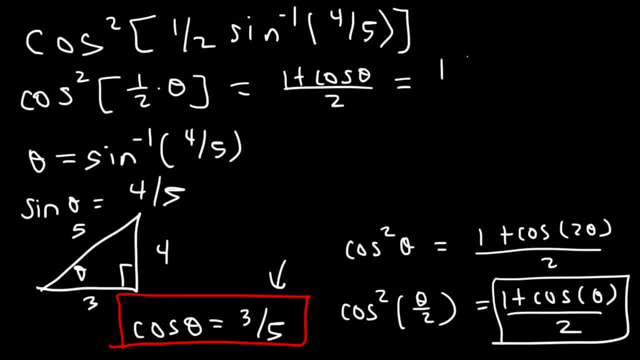 and we already have the value of cosine theta, It's 3 over 5.. So now let's multiply the top and the bottom by 5.. So 5 times 1 is 5.. 3, fifths times 5 is just 3.. And 2 times 5 is 10.. 5 plus 3 is 8. 8 over. 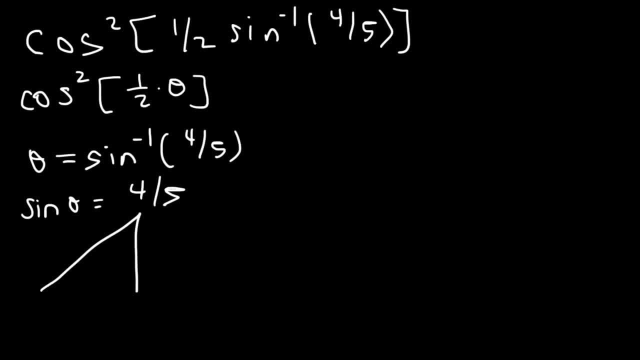 And arc sine is positive in quadrant 1.. So we have a right triangle in quadrant 1.. And sine is opposite over hypotenuse. The missing side is 3.. Now we need the value of cosine, theta. Cosine is adjacent over hypotenuse. 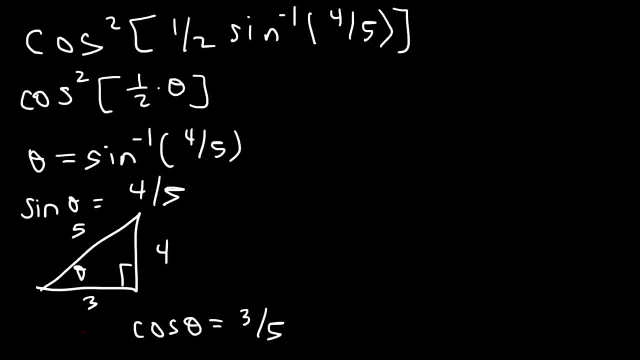 So cosine theta Is 3 over 5.. And we'll use this soon. So right now we need to use the half angle formula Or we can use the power reducing formula. Now we know that cosine squared theta is 1 plus cosine 2 theta divided by 2.. 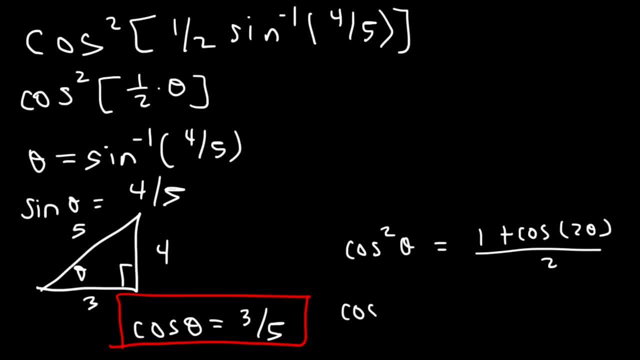 So if we divide this angle by half and get cosine squared theta over 2, which is what we have here- Then all we're going to do is divide this angle by half. I mean not by half, but by 2.. 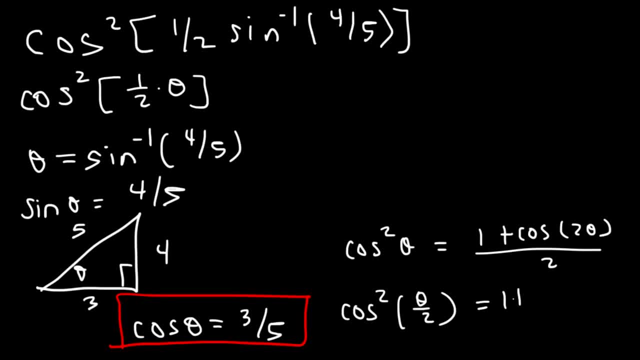 So that will be 1 plus cosine theta over 2. And this is the equation that we need to use. So 1 plus cosine theta divided by 2. And we already have the value of cosine theta: It's 3 over 5.. 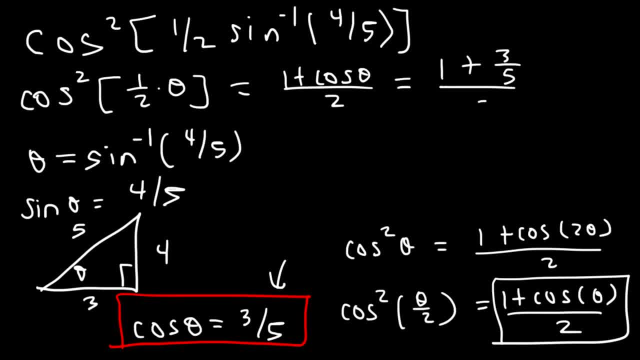 So now let's multiply the top and the bottom by 5.. So 5 times 1 is 5.. 3, fifths times 5 is 3. And it's 4.. So we're left with 2.. 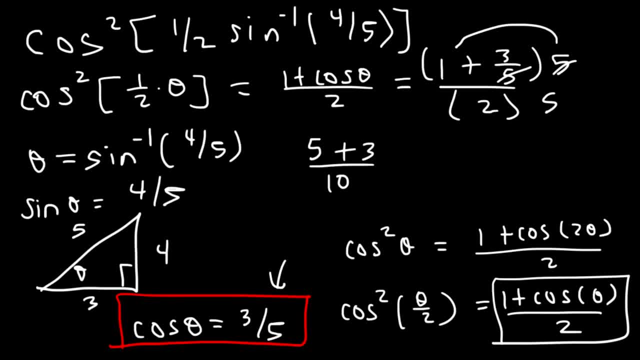 3. fifths times 5 is just 3, and 2 times 5 is 10.. 5 plus 3 is 8,. 8 over 10 reduces to 4 over 5.. And so this is the final answer. 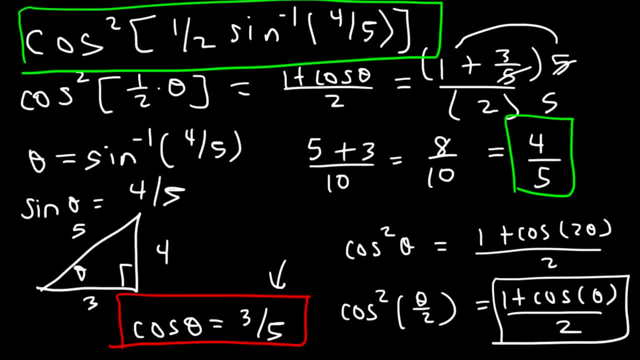 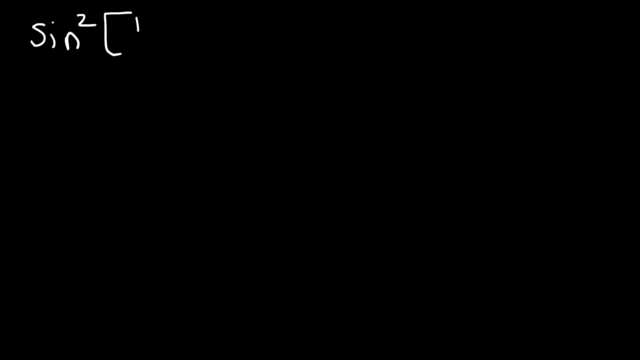 So this entire expression, it's equal to 4 over 5.. Let's try one more problem: Sine squared 1, half arc, cosine 7 divided by 25.. So let's figure this out. So we need to use the formula sine squared 1, half theta. 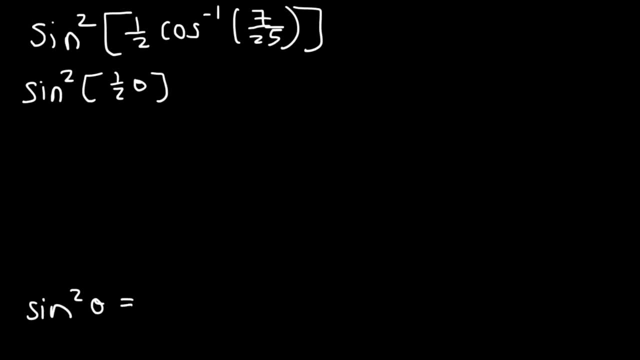 Now we know that sine squared theta is equal to 1 minus cosine 2 theta over 2.. So if we divide this by 2, then we should divide that by 2.. So sine squared theta divided by 2 is going to be 1 minus cosine theta divided by 2.. 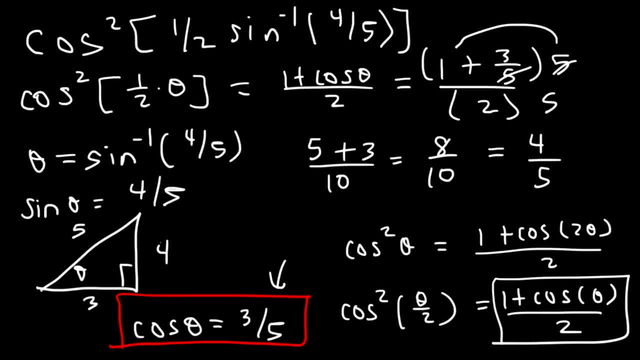 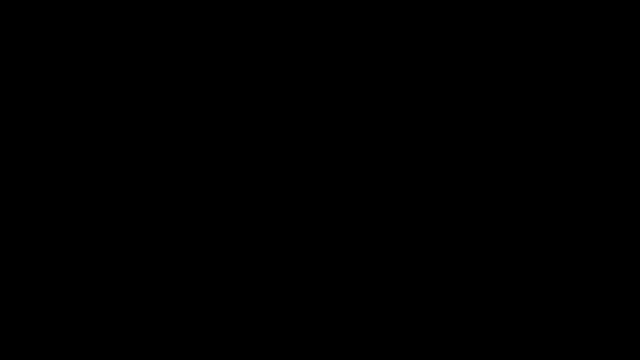 10 reduces to 4 over 5.. And so this is the final answer. So this entire expression: it's equal to 4 over 5.. Let's try one more problem: Sine squared 1 half arc. cosine sine squared. 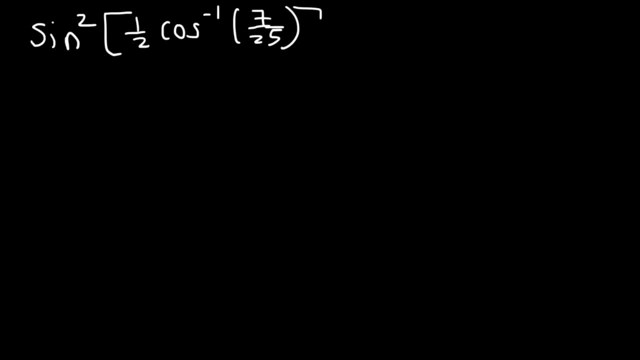 into negative 2.. Thisimet failures Alright. so very briefly, here's the solution for the by-ard problem. Siny squared theta divided by 2 is equal to I minus cosine 2 theta over 2.. So if we divide this by 2, so the is equal to the a minus cosine 2 theta over 2.. So we 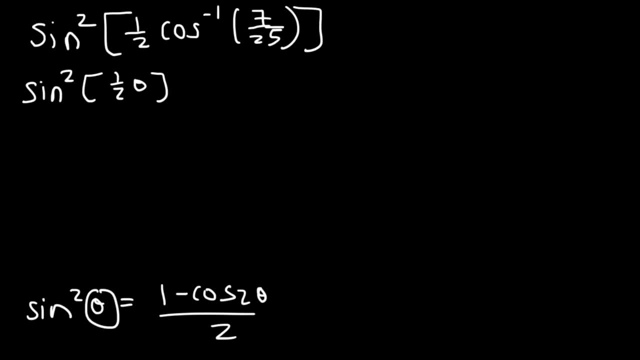 do sine squared one half theta, one sine squared theta divided by 2.. Sine squared theta divided by 2 is going to be 1 minus cosine 2. samen with sine squared that will give us That's going to be negative 1 minus cosine 2 theta over 2. so e at minus. 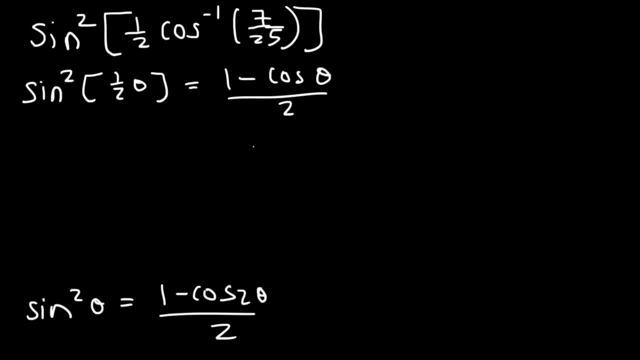 3 on the top left. So now, what do we need to do? We need to do thelk smack and form equals not zero in the denominator, but more zero in the denominator. so even if theta divided by two, So if you divide this by two, divide this by two, which just gives you. 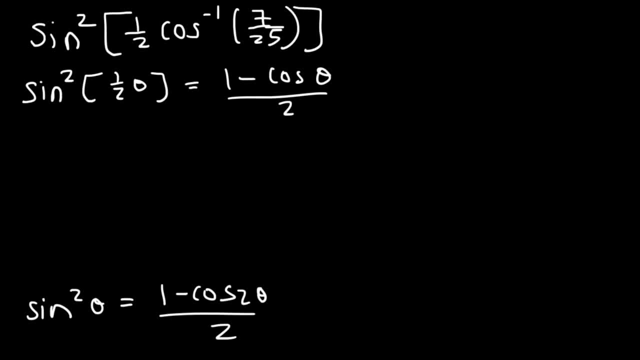 theta. Now theta is arc cosine. So if theta is arc cosine seven over 25, then cosine theta is seven over 25.. So we don't need to draw a triangle because we have the value of cosine theta. So this becomes one minus seven over 25 divided by two. Now let's multiply the top and 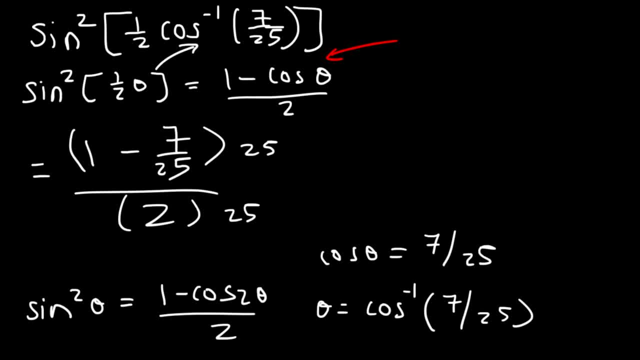 the bottom by 25.. So 25 times one is 25, and then seven over 25 times 25, that's seven Two times 25 is 50.. 25 times 25 is 25.. 25 times 25 is 25.. 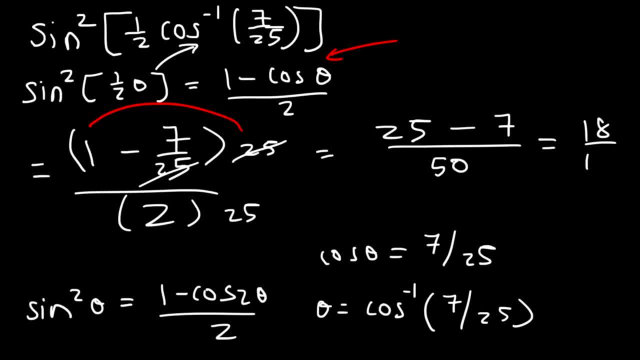 25 minus seven is 18.. And 18 over 50,. if you divide both numbers by two, this will give you nine over 25, which is the final answer. By the way, if you type this in your calculator, it should.